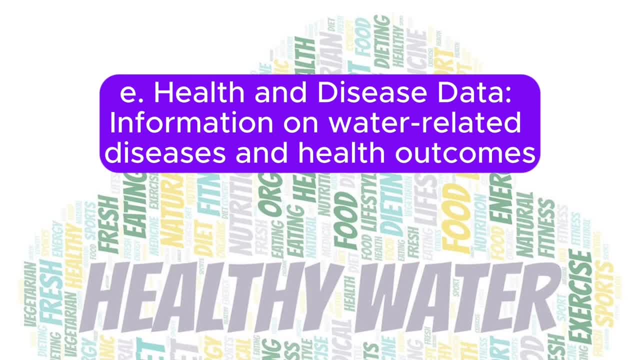 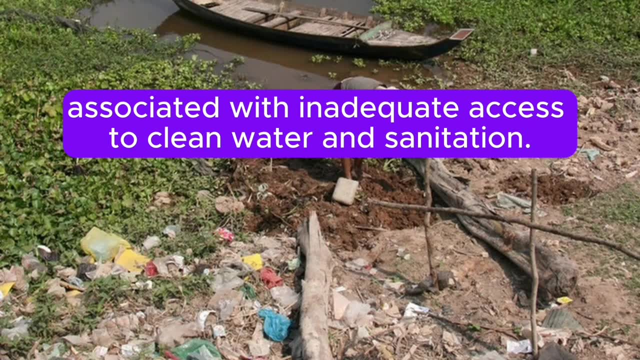 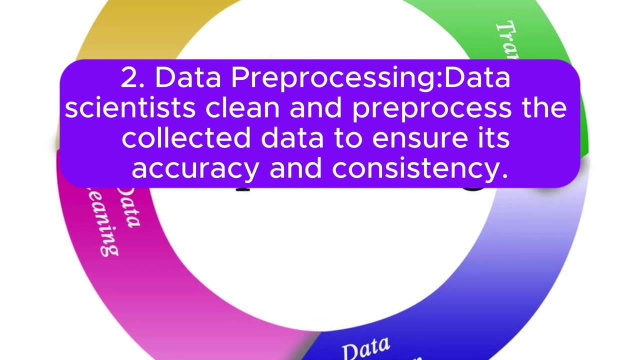 water sources and water quality. e Health and disease data: information on water-related diseases and health outcomes associated with inadequate access to clean water and sanitation. 2. Data prepressing: Data scientists clean and pre-process the collected data to ensure its accuracy and consistency. 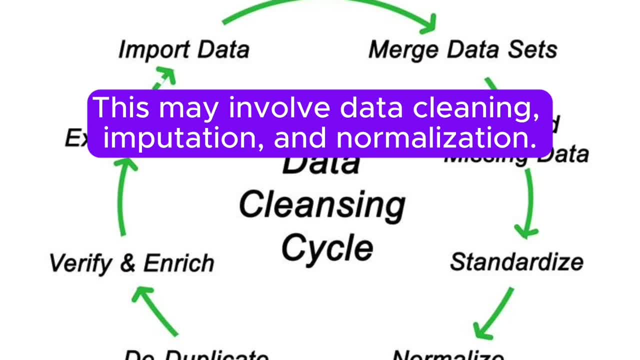 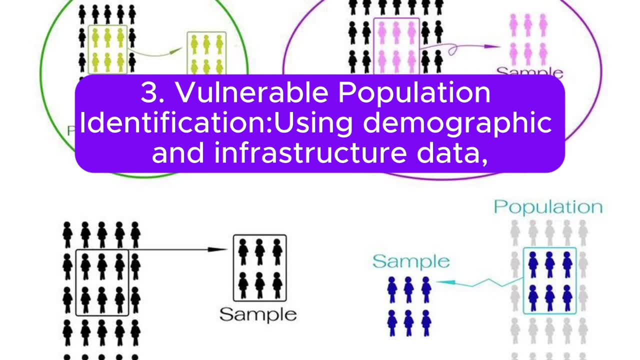 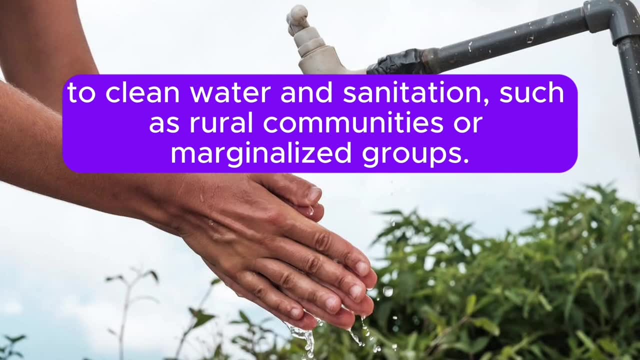 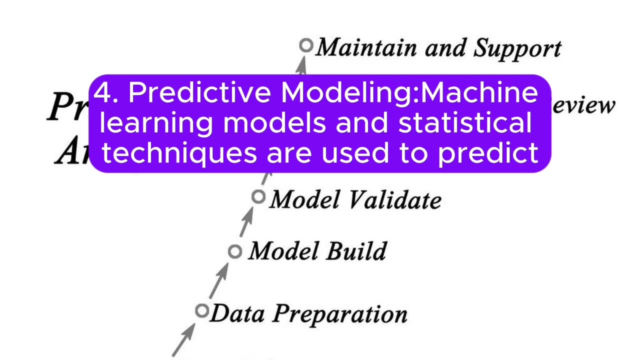 This may involve data cleaning, imputation and normalization. 3. Vulnerable population identification: using demographic and infrastructure data, Data scientists identify vulnerable populations lacking access to clean water and sanitation, such as rural communities or marginalized groups. 4. Predictive modeling: Machine learning models and statistical techniques are used to predict. 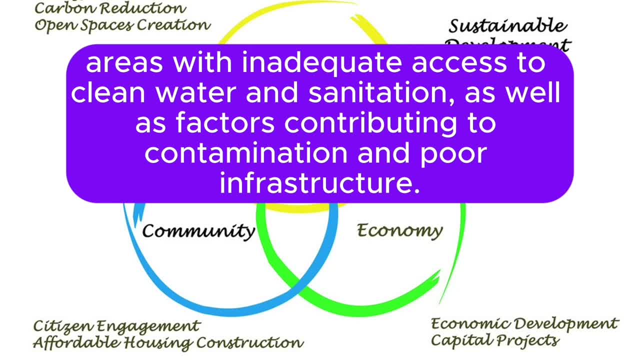 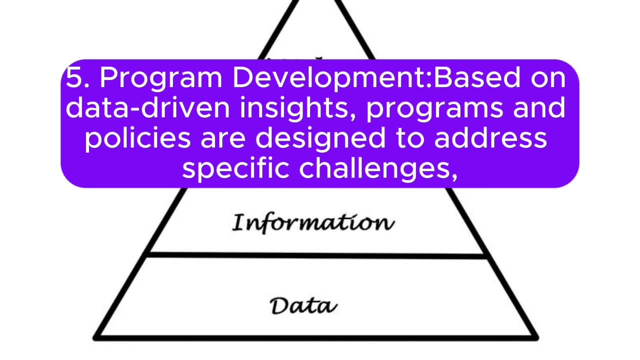 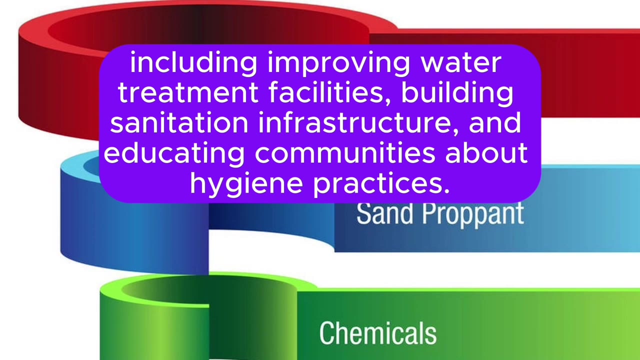 areas with inadequate access to clean water and sanitation, as well as factors contributing to contamination and poor infrastructure. 5. Program development based in data-driven insights. Programs and policies are designed to address specific challenges, including improving water treatment facilities, building sanitation infrastructure and educating communities about. 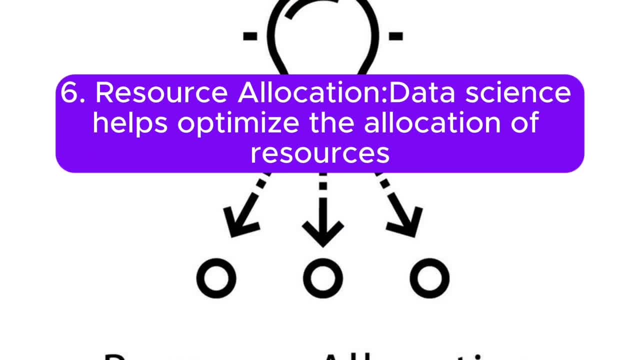 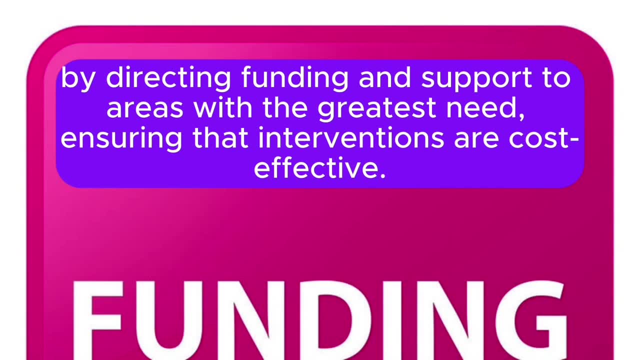 hygiene practices. 6. Resortialization: Data science is playing a critical role in addressing pollution in carbohydrates and marsh monks in local city- 소리 sai. Data science helps optimize the allocation of resources by directing funding and support to areas with the greatest need, ensuring that interventions are cost-effective. 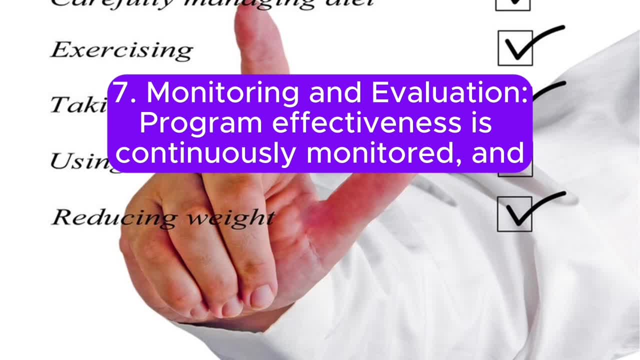 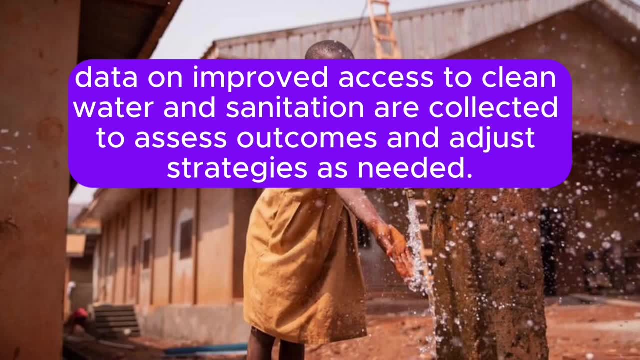 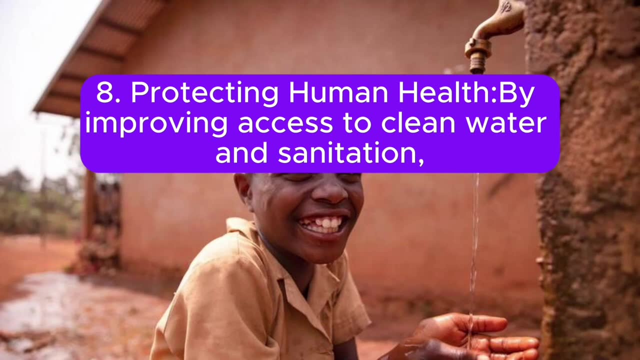 home and Kia set self-styling provision lessons. 7. Monitoring and evaluation: Program effectiveness is continuously monitored and data on improved access to clean water and sanitation are collected to assess outcomes and adjust strategies as needed. ou 기p diversity de Brusseles, Kaipapas and línea Bal 열�ion top reviews and Forschion. 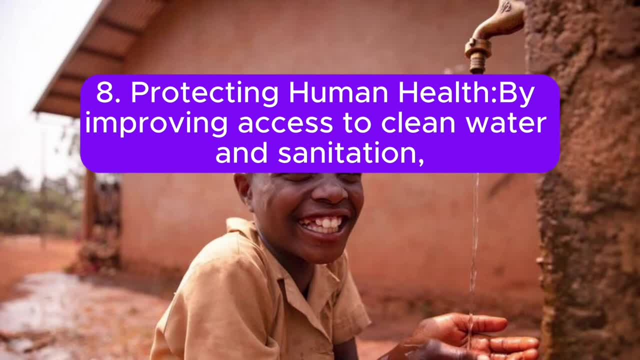 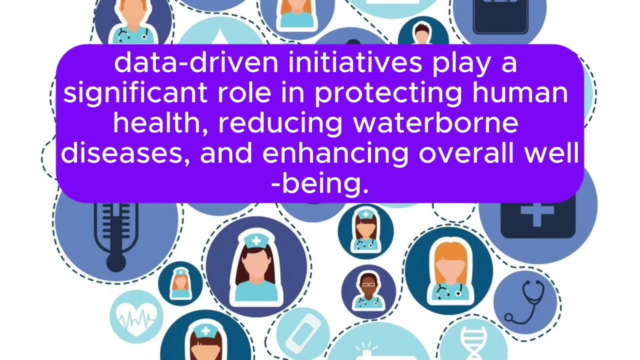 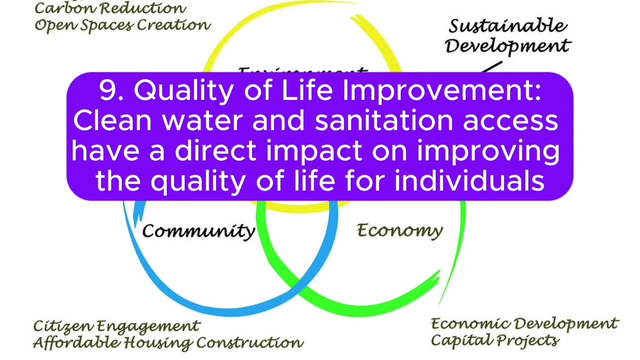 human health by improving access to clean water and sanitation. Data-driven initiatives play a significant role in protecting human health, reducing waterborne diseases and enhancing overall well-being. 9. Quality of life improvement. Clean water and sanitation access have a direct impact on improving the quality of life for individuals and communities, contributing to